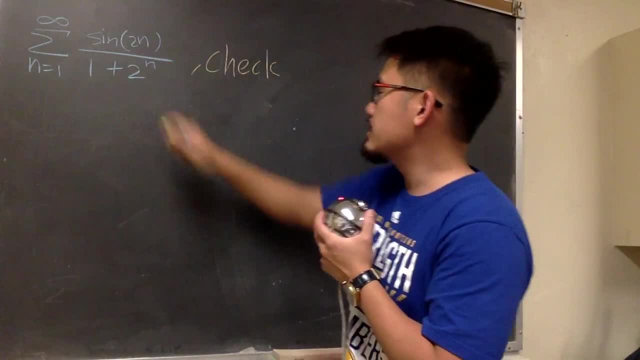 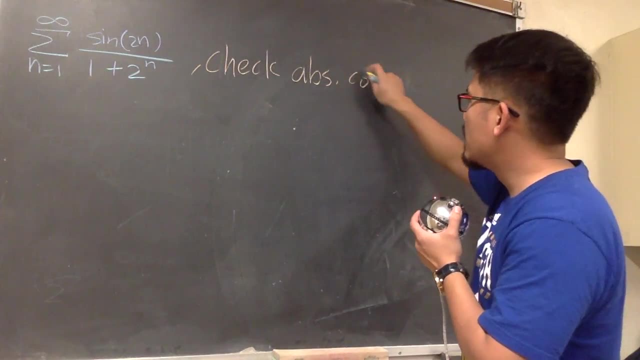 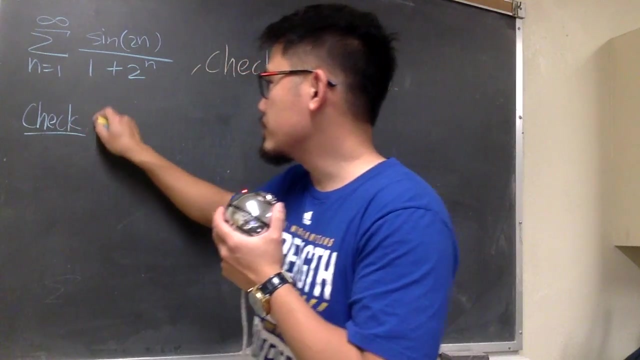 So let me tell you, instead of working with this, I will check the absolute value version of the original. So that's checking for absolute convergence, Convergence or not, And let me show you how it works. So let me just write it down. we are just going to check. 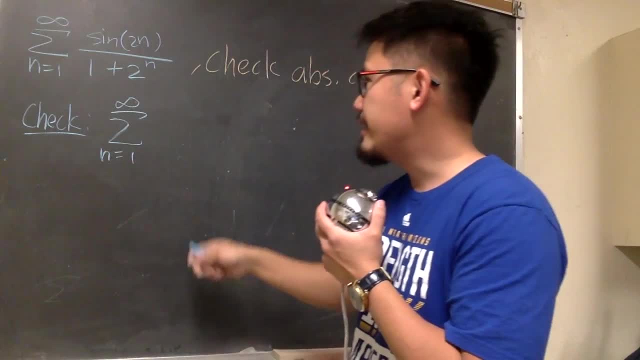 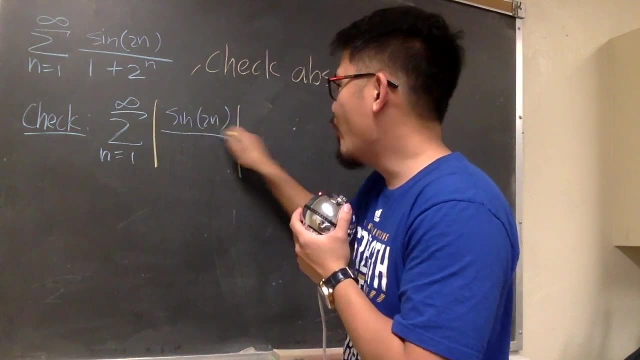 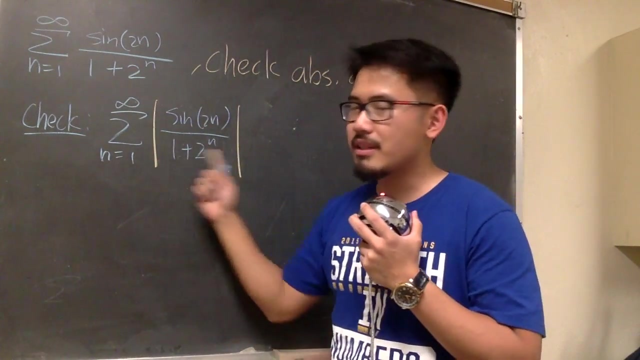 Let me put down sigma where n goes from 1 to infinity and I will put down an absolute value and then we'll put down this inside sine of 2n over 1 plus 2 to the n. If we have this absolute value and if this converges, of course the original converges as well. 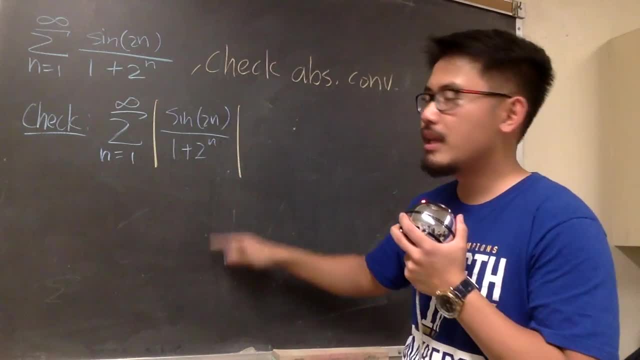 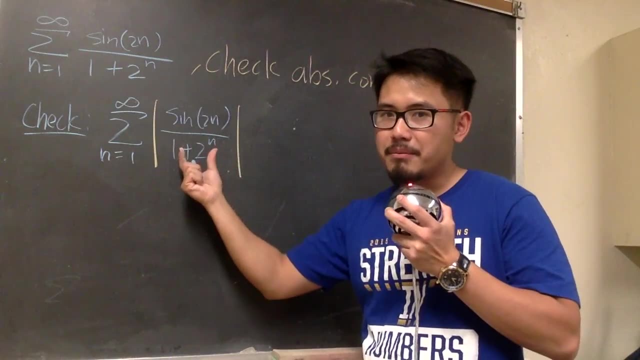 And the good thing right here is that when we have this absolute value, we have this sine factor inside And once again, this sine factor it cause the expression inside, Sometimes it's being negative, sometimes it's positive, but it's okay. 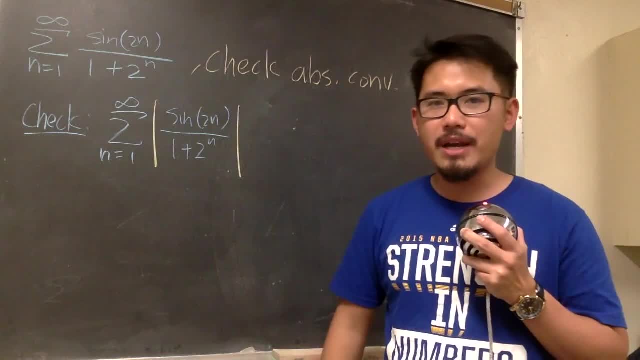 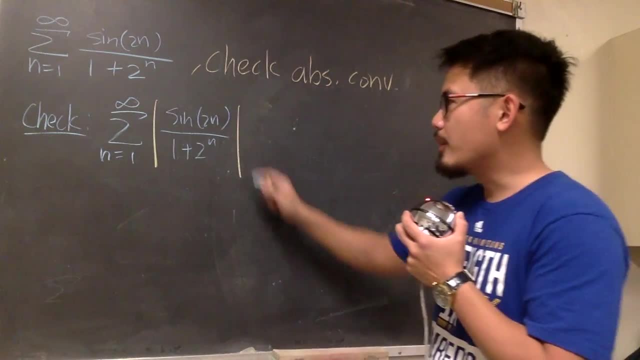 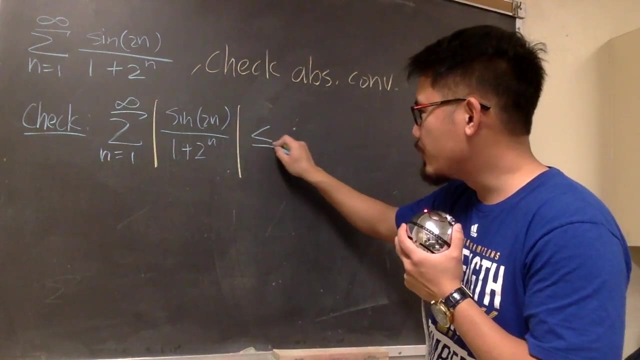 The absolute value will make everything positive inside right. Furthermore, we know sine of any angle has the maximum value 1.. So, on the numerator, we know this is always going to be less than or equal to 1.. So I can write this down: this is less than or equal to. we have the 1 on the top. 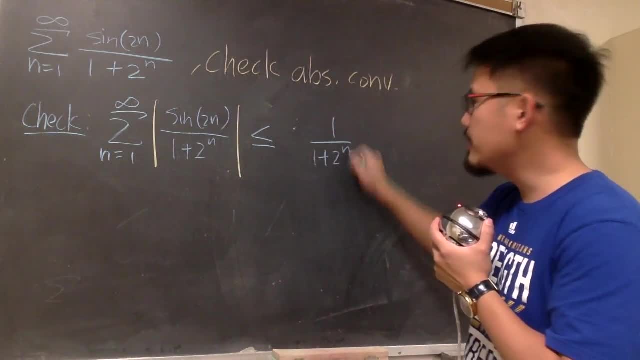 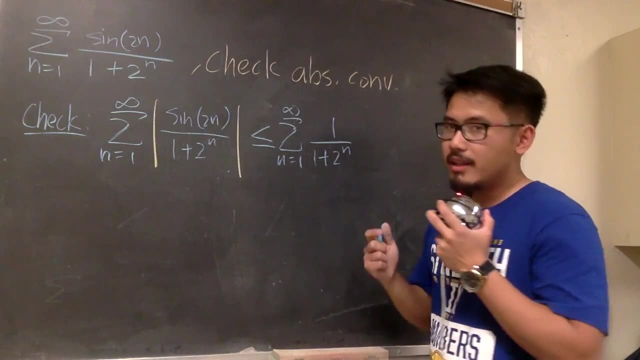 And then the denominator stays the same: 1 plus 2 to the n. And also let me write down the sigma notation, and it goes from 1 to infinity. And once again, absolute value of sine of 2n is less than or equal to 1.. 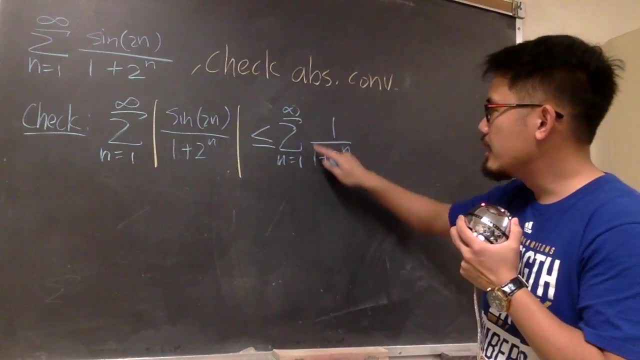 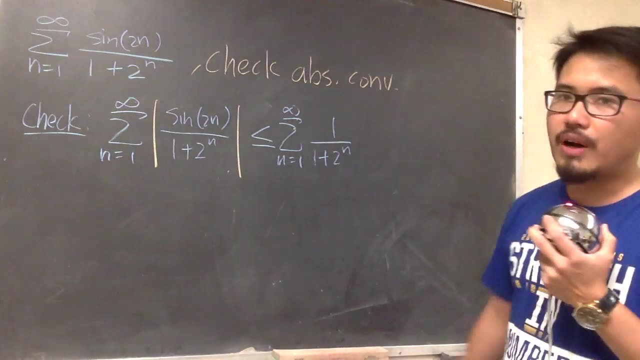 That's how I was able to build this up, And you see here, 1 over 1, plus 2 to the n. This is always positive. now I don't need the absolute, the value, anymore, And now we just have to work with this. Well, if you ignore the 1, 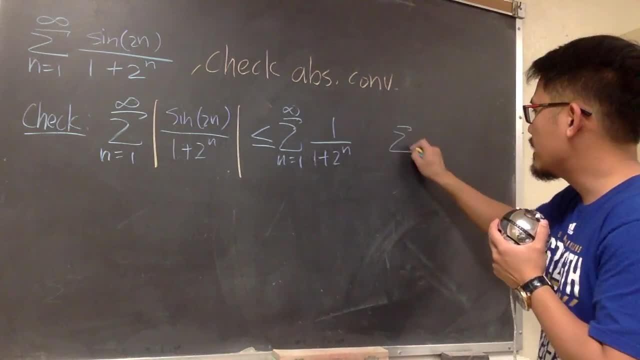 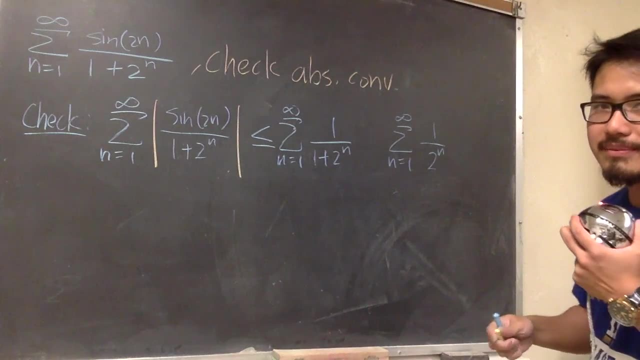 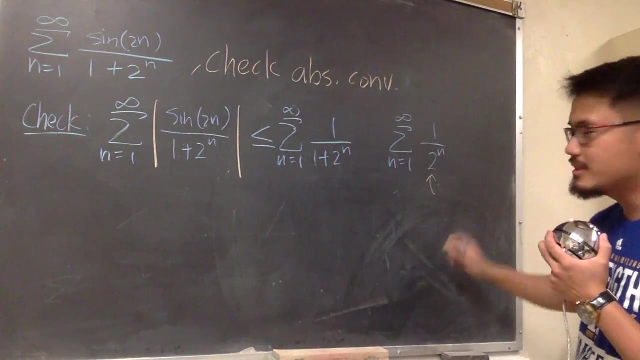 in the denominator. you are looking at this as sigma when n goes from 1 to infinity, and then we just have 1 over 2 to the n instead. Do we know much better about this? Yes, we do. We certainly do, because this is a geometric series. we know r is equal to 1, half We can. 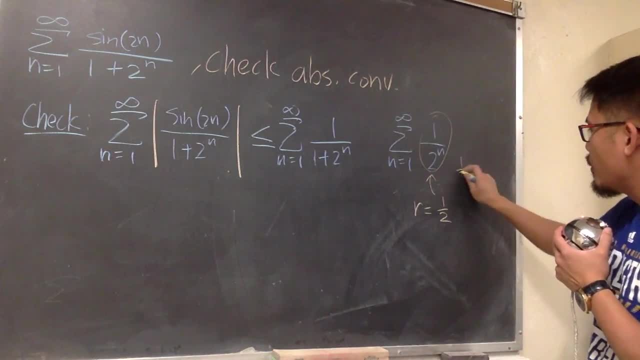 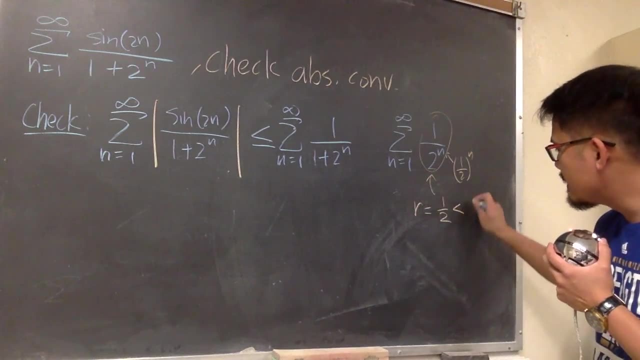 look at this as 1 over 2 to the nth power right. So r is 1 half. Well, 1 half is less than 1, and from the geometric series we know this converges. All right, and now let's. 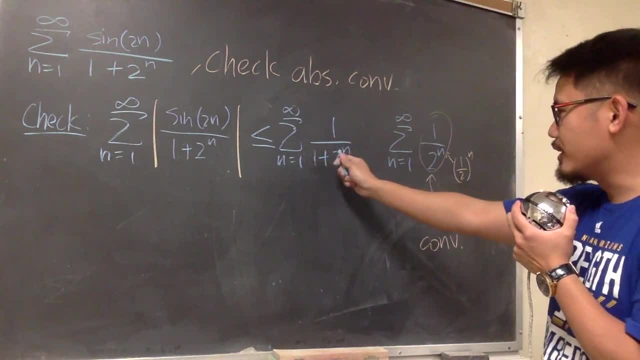 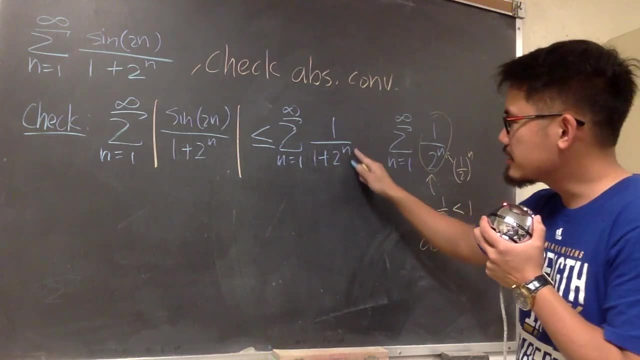 talk about. what good does this do? Can we build any connection between this 1 and that 1?? The only thing different is that we took away the 1 in the denominator. Look at this. Originally, this part here, this is bigger than that denominator, right? But when you? 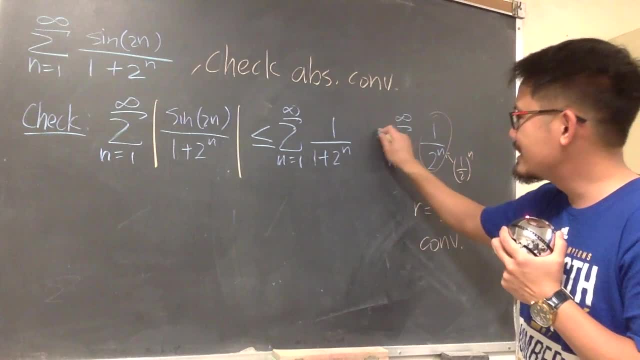 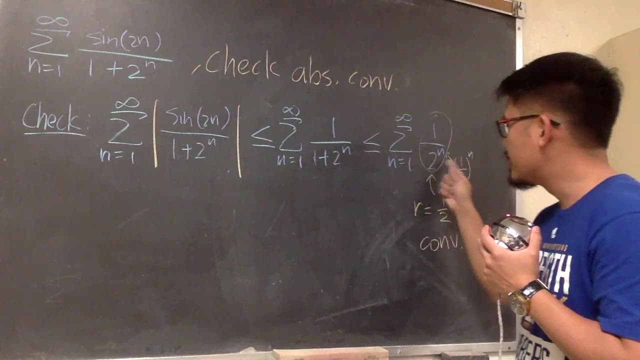 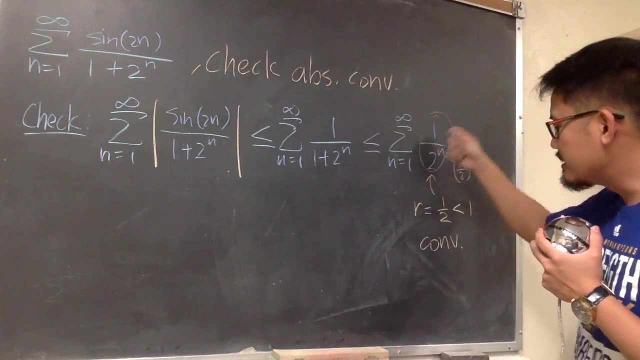 have the 1 over this. it's going to be smaller than this 1.. So let me just put down less than or equal to: The bigger the denominator, the smaller the reciprocal is. So now we know this is less than or equal to that and this is a convergent, which is the finite value. 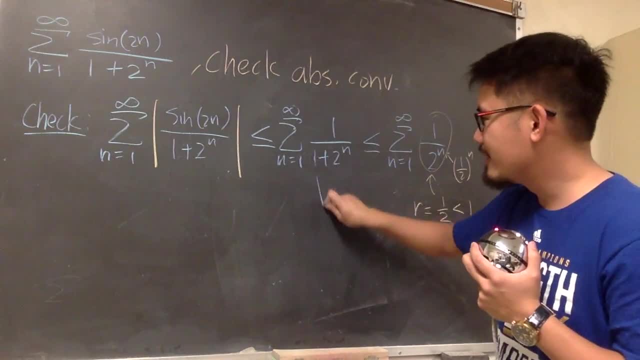 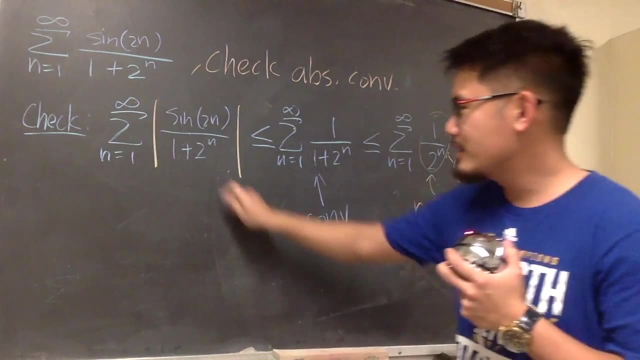 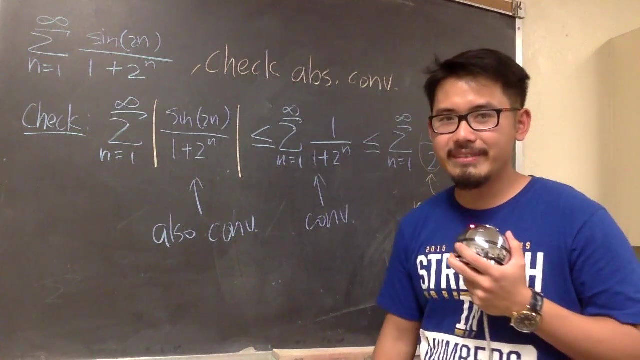 We can also conclude that this is 1 over 2. This is a convergent right, So this right here converges, And likewise this is less than a convergent, So of course this at the end also has to converge. 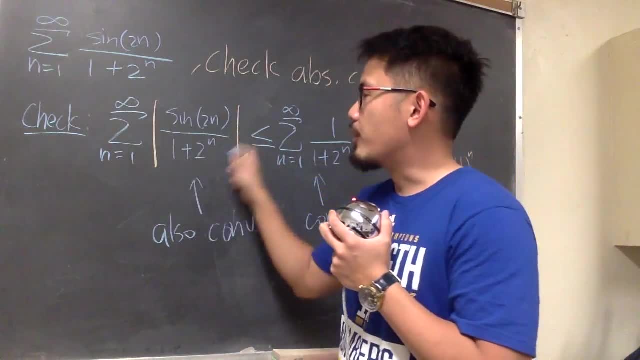 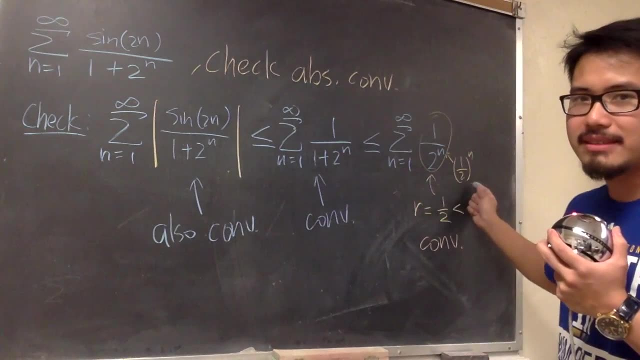 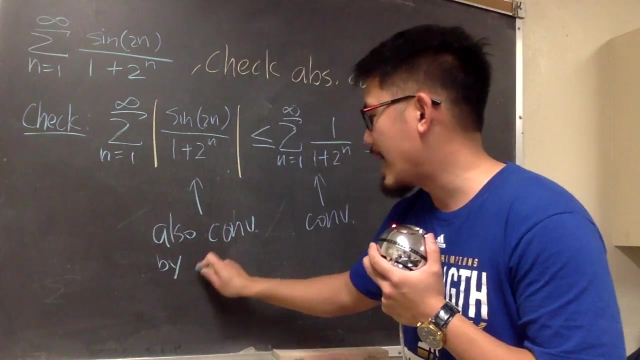 So now here's the conclusion: The absolute value version of the very original. this right here, converges by direct comparison test. right, Because we have the inequality, So let me just write this down. Also converges by direct comparison test, And likewise. 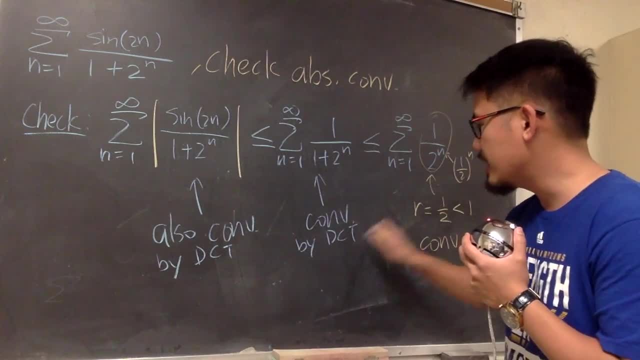 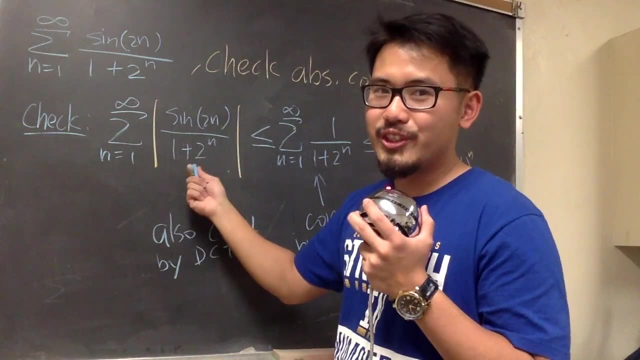 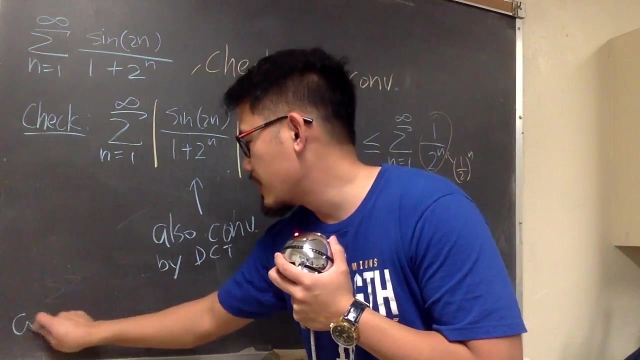 this is also a convergent by direct comparison test, And I'm just going to tell you if the absolute value version right here converges. when you don't have the absolute value version, of course, it converges as well. So now I can just write down the final conclusion here. 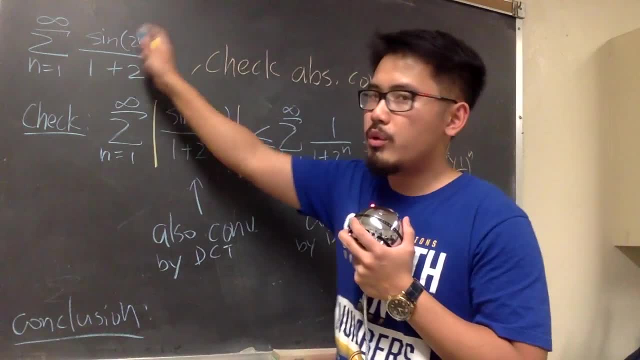 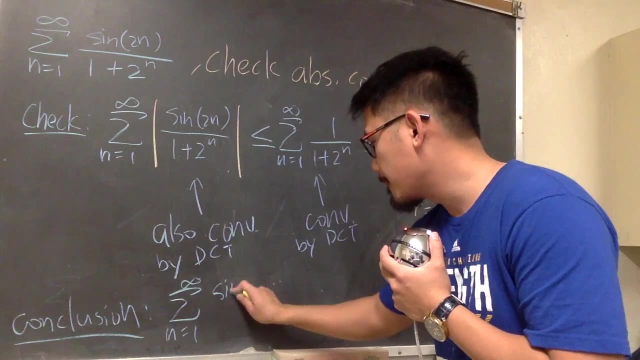 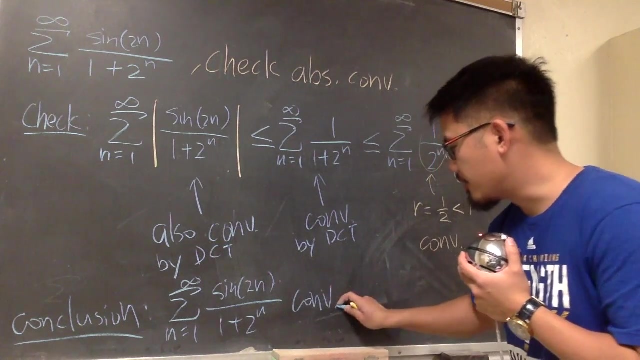 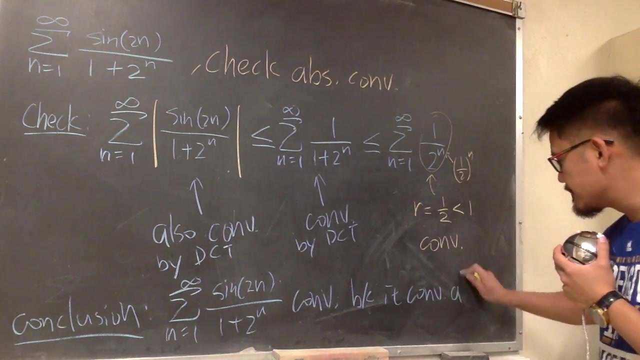 You always write down the conclusion And then put down the final conclusion And then put down the very original. And that very original is the sigma where n goes from 1 to infinity sine of 2n, over 1 plus 2, to the n converges because it converges absolutely, meaning the 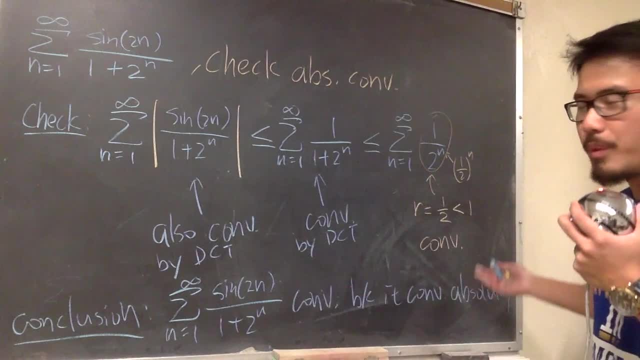 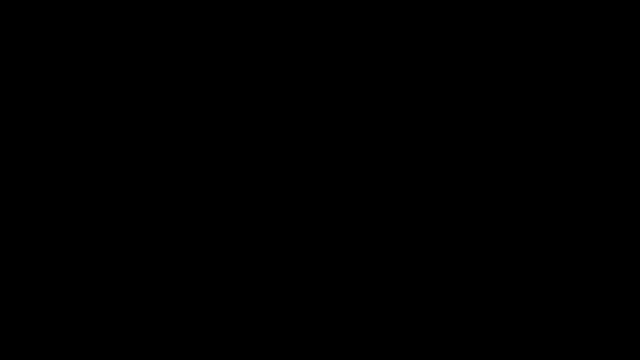 absolute value version of that converges. So this will be it Good argument to show that it converges. That's it.